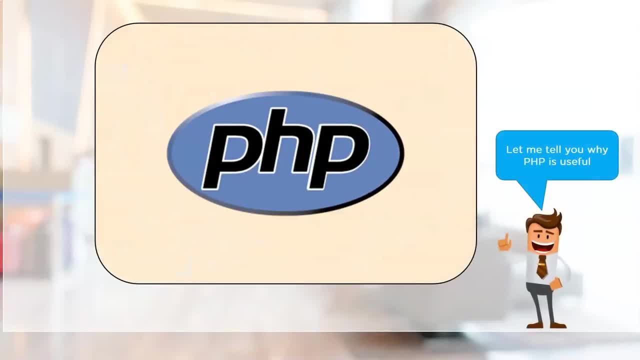 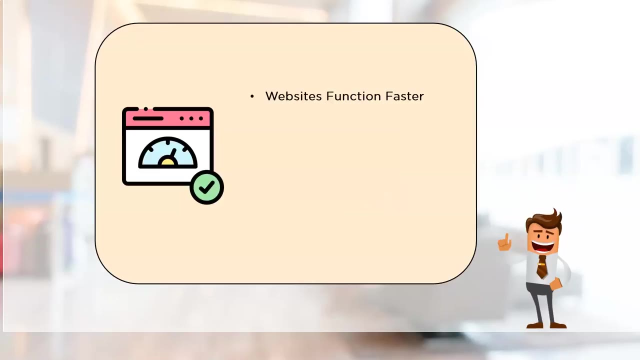 His websites in PHP can solve all of Rob's problems. And guess what? PHP is simple to learn and easier to implement. Let me elaborate on this. PHP is useful in many ways as, first and foremost, it can make the website function faster. It can create dynamic webpages and 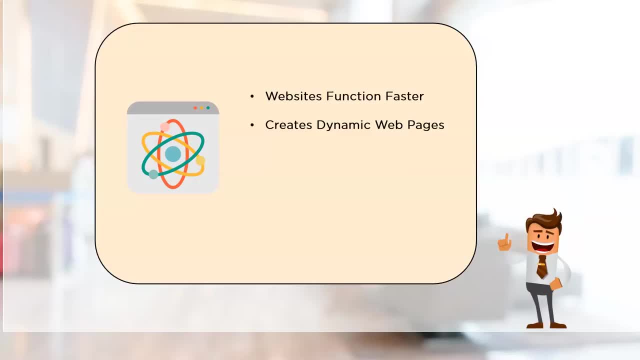 dynamic webpages are what makes a website more interactive. Next, it provides security encryption. It is a cost-efficient website. It can create dynamic webpages, and dynamic webpages are what makes a website more interactive. Next, it provides security encryption. It can. 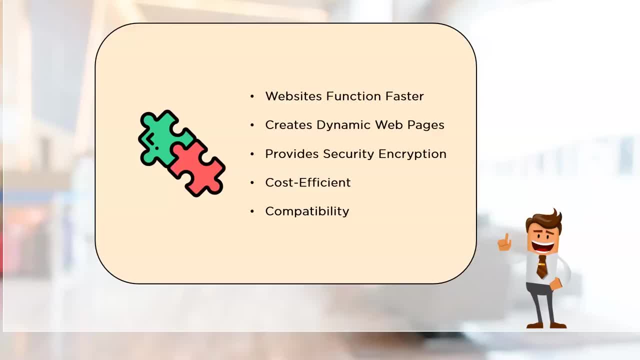 create dynamic webpages, and dynamic webpages are what makes a website more interactive. Next, it provides security encryption. It can create dynamic webpages and dynamic webpages as it works efficiently with different databases and programming languages. And it is platform independent, which means the PHP application can run on any environment. 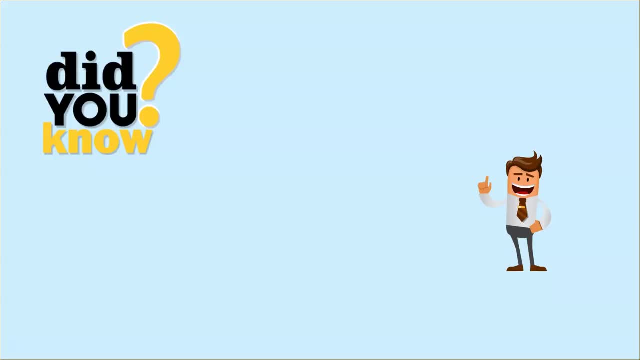 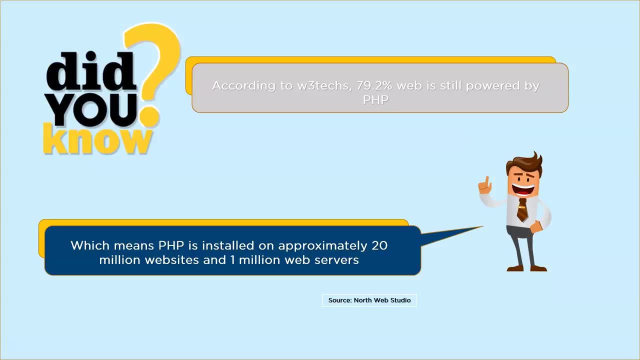 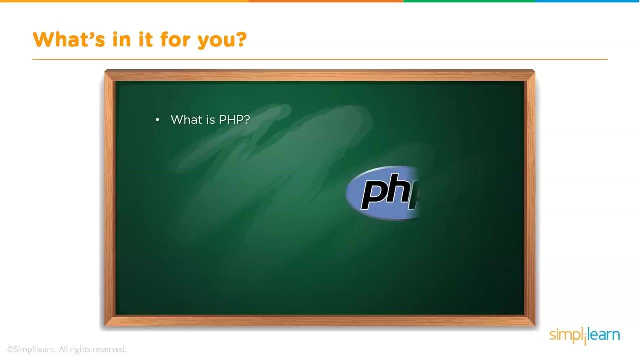 Now, before moving into the details, did you know that 79.2% web is still powered by PHP, which nearly translates to 20 million websites and 1 million web servers? Now, in the future, In this presentation, you'll learn about what is PHP, how does it work, differently from. 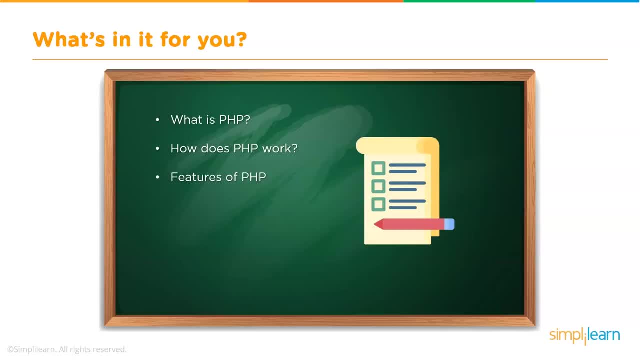 a conventional web page. what are its features? some major companies where PHP is implemented, prerequisites on learning it and, finally, we will have a look at the demo for our first PHP program Now, without further ado, let's get started. 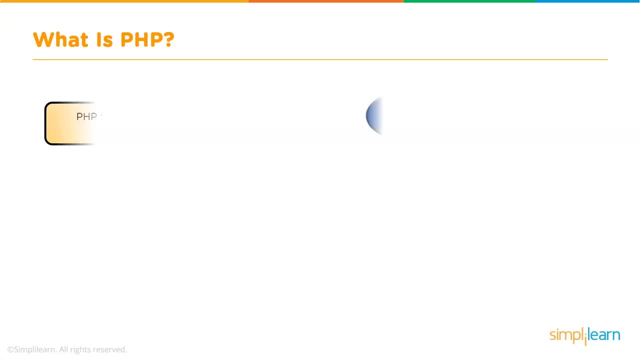 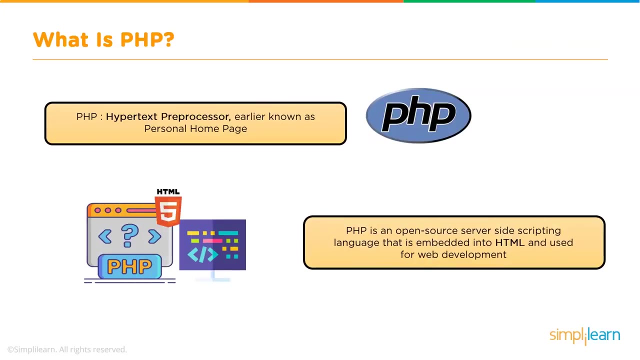 So what exactly is PHP? PHP stands for Hypertext Preprocessor, which is a recursive acronym. It is an open-source server-side scripting language that is embedded into HTML and used for web development. Now, before we get overwhelmed by the technical terms, let me simplify them for you. 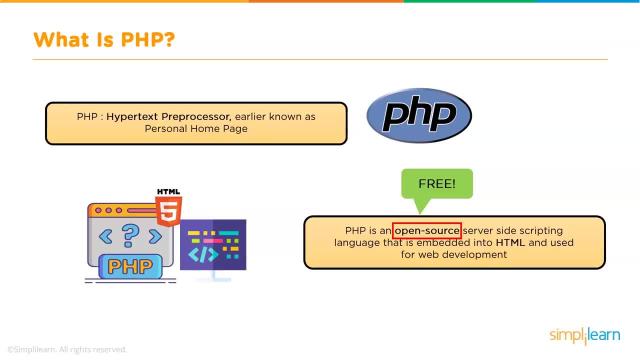 Now for those of you who don't know: open-source is a term for technology, which means it is freely available to everyone, while server-side scripting means that, from writing the code to implementing and processing the code, it is freely available to everyone. 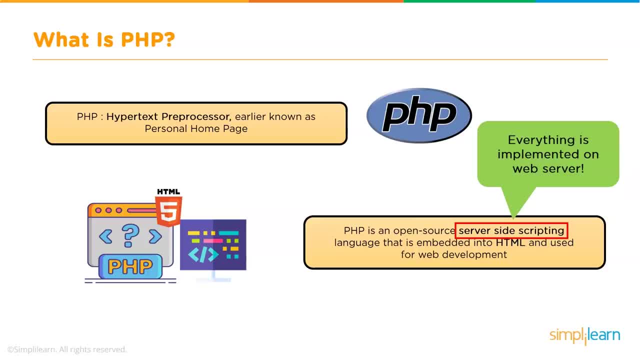 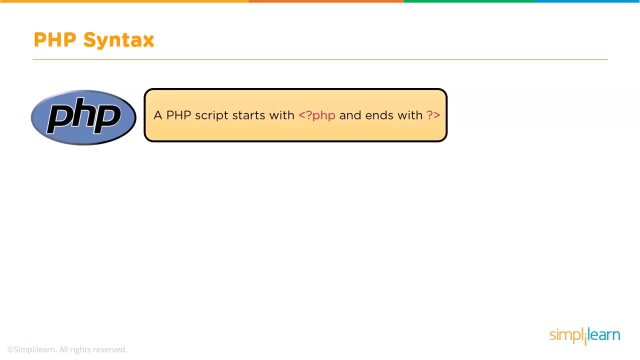 While processing it, everything is done on the server-side, while the user just lays down and enjoys the experience. Now that we know what PHP is, let's see how a PHP script looks like. As you can see on the screen, this is the syntax of PHP. 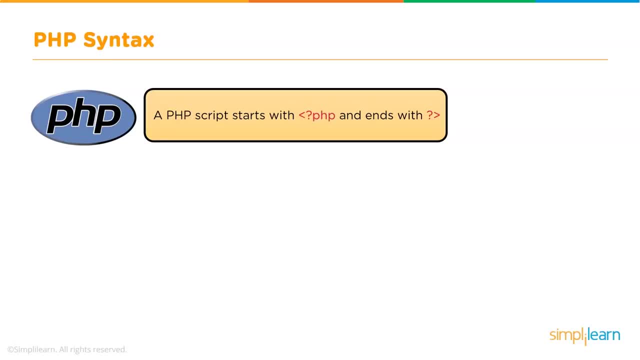 It opens with an angled bracket- question mark- PHP and ends with a question mark and an angled bracket, while the code comes in between them. Now, as you can see, this is the syntax of PHP. As you can notice, this is very similar to how HTML codes are written. 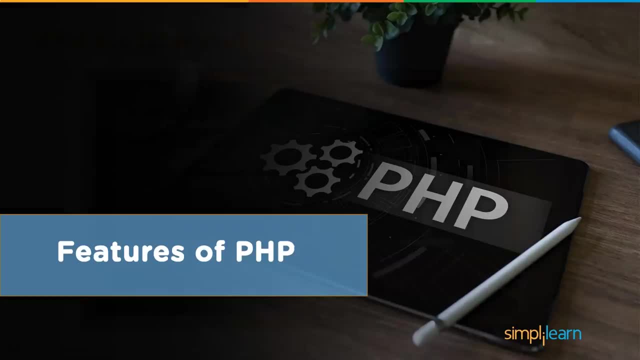 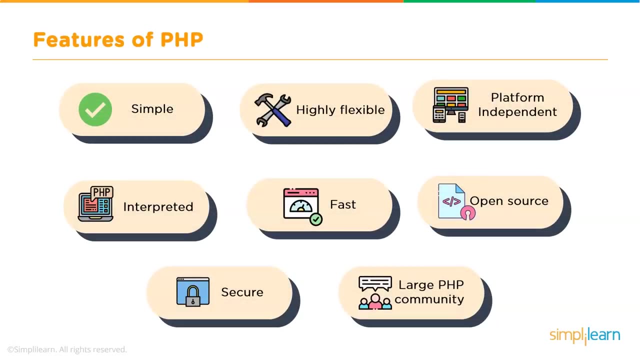 Now let's have a look at some features of PHP. Now, while PHP being a very diverse and feature-rich language, some of its main features are listed here. Let us try and understand them one by one. First is simple. Now, this feature comes as a good news to new learners, since PHP is simple and hence 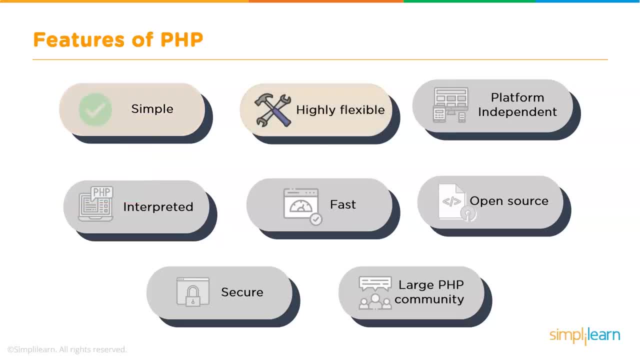 an easy-to-learn language. Next comes flexibility. PHP is a highly flexible language. In conventional webpages, even the smallest of changes have to go through the developer, who changes the code to implement them, while PHP gives you the flexibility to make small. 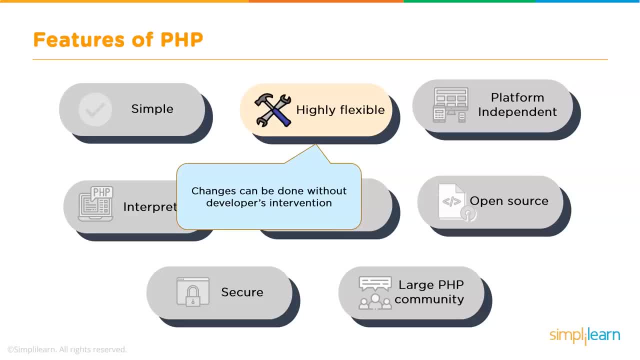 changes without the intervention of the developer itself. It is also platform-independent, which means it does not require any special plugins to run and can basically run on any environment. Next is interpreted: PHP is an integrated language. PHP is an interpreted language and does not compile the entire code, hence taking less. 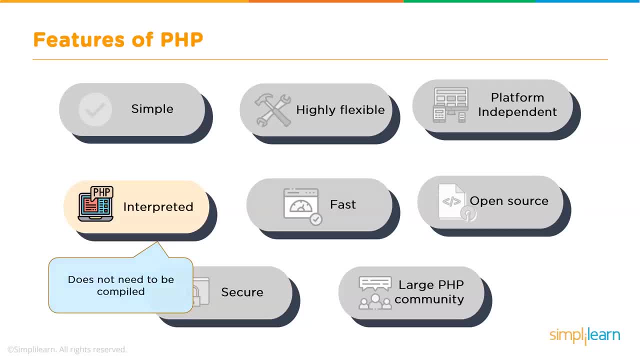 time, Which takes us to our next feature, that is, fast. Websites developed in PHP are faster. This is why developing dynamic websites using PHP is considered as the best option. As discussed earlier too, PHP is called as an open-source language, which means it is. 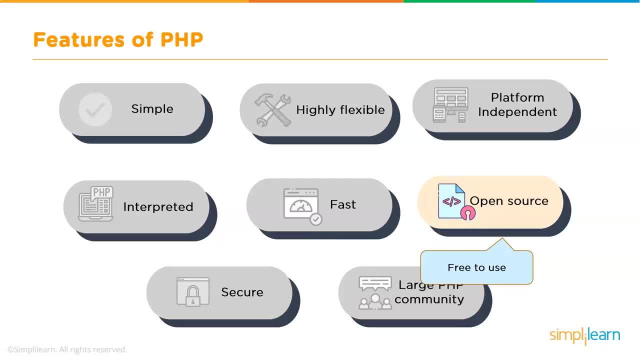 free to use and implement. Next feature is security. Next feature is security. The language consists of a few built-in frameworks that provide benefits like encryption and hence, protection from cyberattacks. Next is a large PHP community. Since PHP is an old language, it has grown up to a large community, which is very helpful. 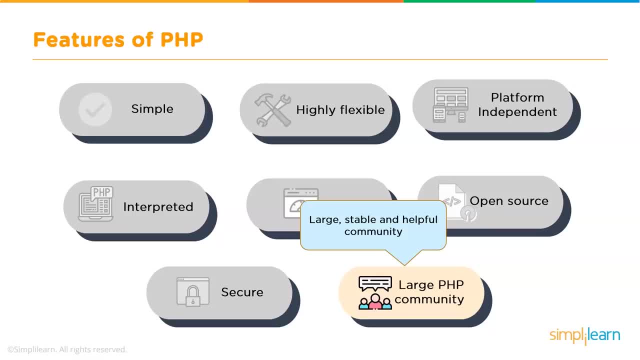 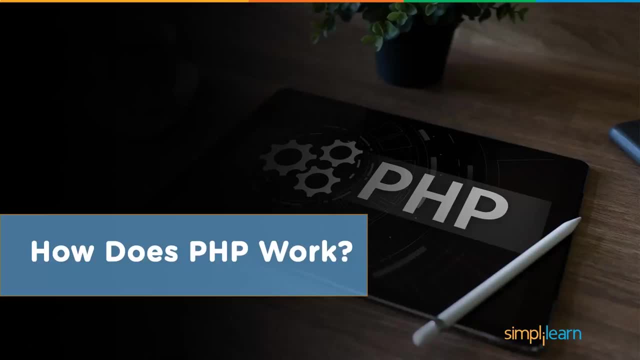 and makes the language more stable. That was all about features of PHP. Moving forward, let us discuss the workflow of a PHP webpage. How does a PHP community work? So, for a better understanding, let us first see how a basic HTML page functions. 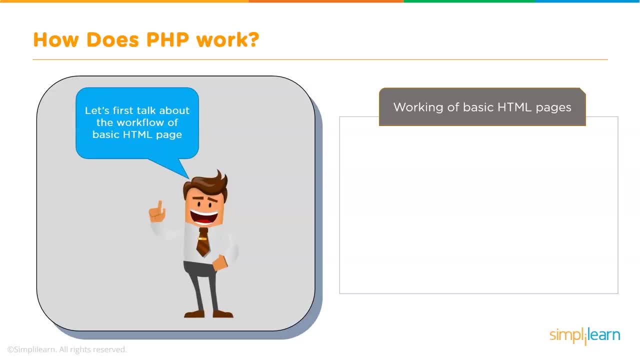 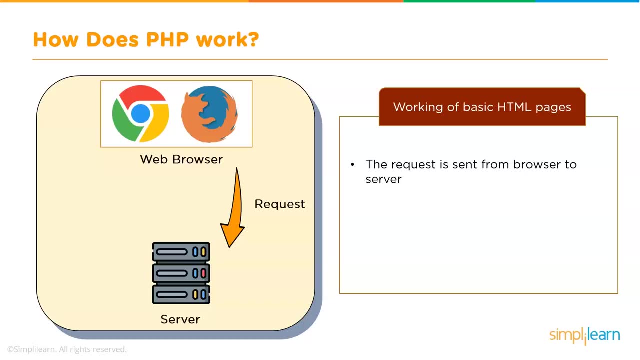 In the basic HTML workflow, when you open a website on your browser, a request is sent from the browser to the server, and the server then returns the requested page stored on it back to the browser. Now that's it, No matter what device or what purpose you open the website for. 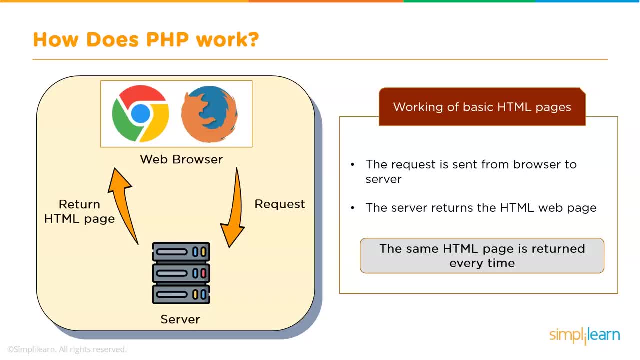 The server then returns the requested page stored on it back to the browser. Now that's it. No matter what device or what purpose you open the website for, The page returned is always the same. The page returned is always the same. All you can say is static. 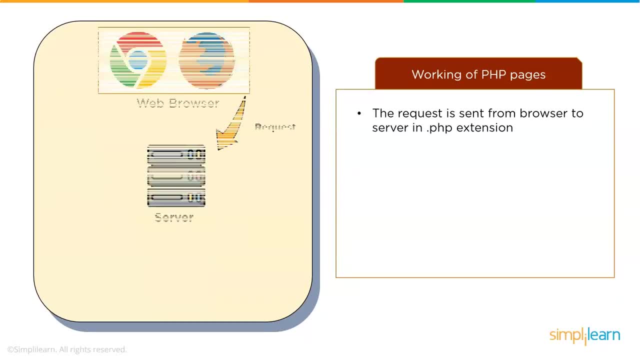 Now what PHP does. different is when you open a website developed in PHP, a request in php extension is sent to the server. Into the server, there exists a PHP interpreter which recognizes the php file and interprets it. Based on the request from the browser, it pulls out data from its database and file. 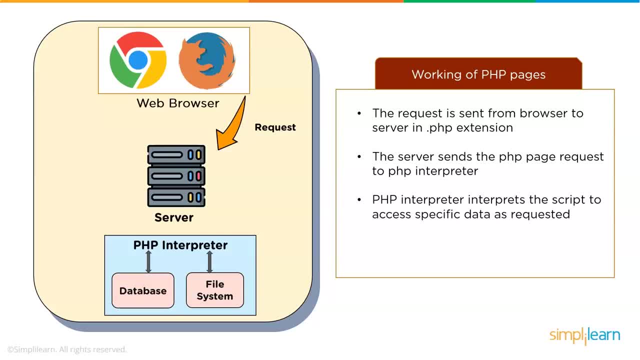 systems and returns an output and returns a HTML page personalized according to the user. Now let me give you an example to make it more clear. When you login to your account on Rob's new ecommerce website made on PHP, it takes your unique request to the server and shows you products based on your past preference. 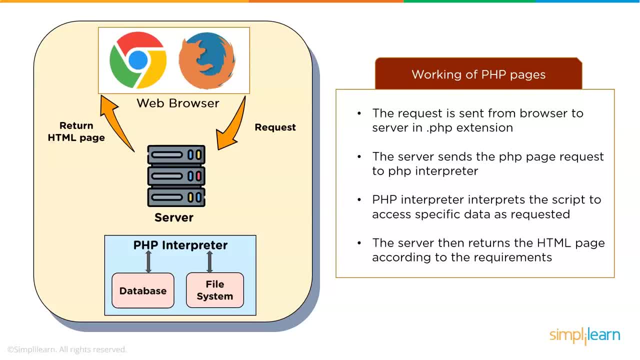 and liking, instead of showing you the exact same page every time. This makes the website dynamic and more interactive to the user. Also, guys, before moving forward, if you are enjoying this video, please give a thumbs up and subscribe to Simply Learn for more such content. 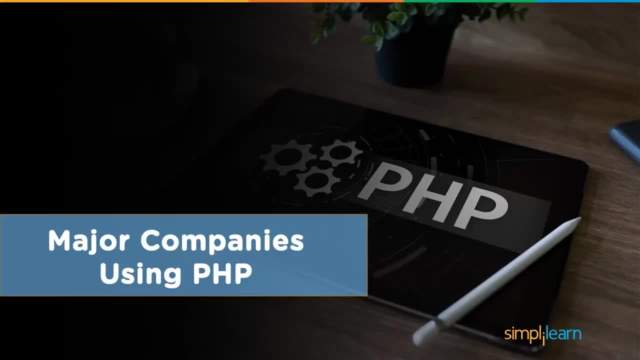 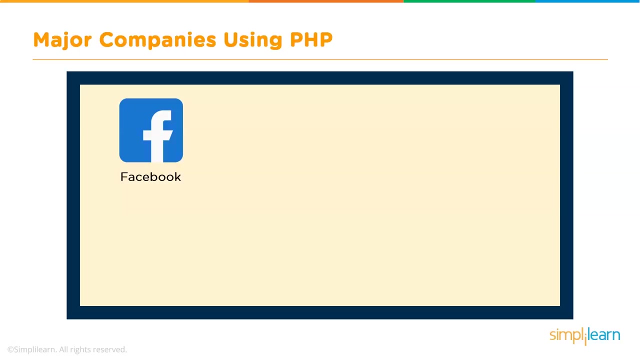 So that was all about the workflow of PHP. Let us discuss the companies using them. Many companies have reached great success by implementing PHP into their websites. Let me list down a few of them. First comes Facebook, the biggest social media platform. Did you know that Facebook was created entirely on PHP? 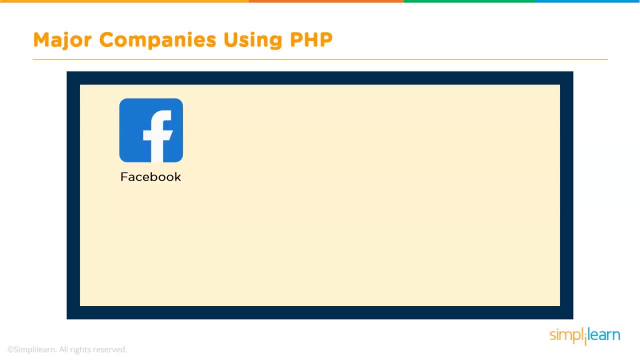 And according to the website SimilarWeb, PHP is visited by users for nearly 22 billion times per month. This means the social media platform has to deal with huge traffic volumes, And PHP helps the website with this. Before moving to the next website, a quick question for you guys. 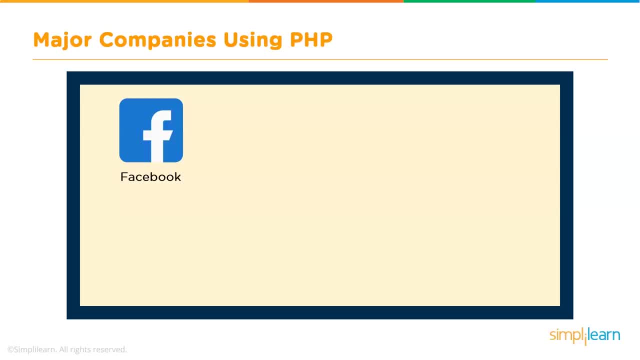 What is the one site everyone goes to for information? Correct, it's Wikipedia. And guess what? It's written in PHP too. Now, platforms like WordPress, which are used to create beautiful websites, itself are also based on PHP, And blogging and social media channels such as Tumblr, and even multi-service platforms. 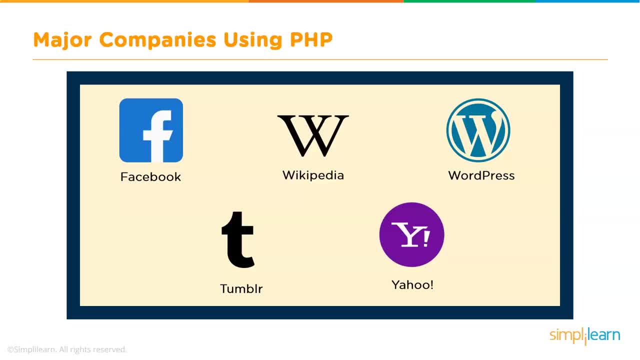 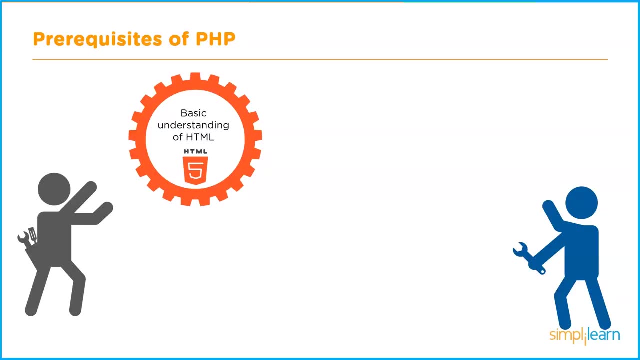 like Yahoo, which face huge amounts of data traffic every day, uses PHP to function. So now that I hope you're more motivated to learn PHP, let us look at some of the prerequisites of learning it Now, since PHP scripts, as already discussed, are embedded into HTML codes. a basic understanding. 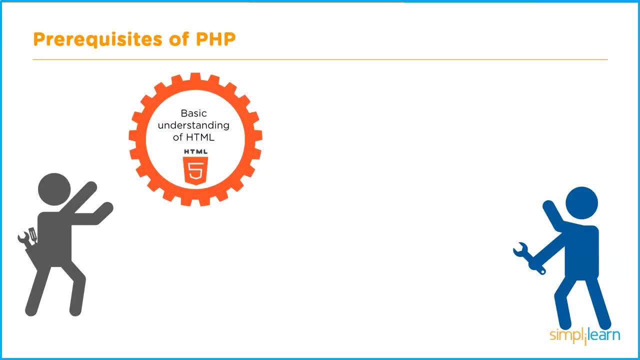 of HTML comes naturally as a prerequisite. Again, a website cannot be complete without the implementation of CSS. Hence, a basic understanding of CSS is also a must. Next is basic knowledge of programming language. Now, this is not necessarily a prerequisite, But if you have basic knowledge of programming fundamentals, such as PHP, you can do it without. 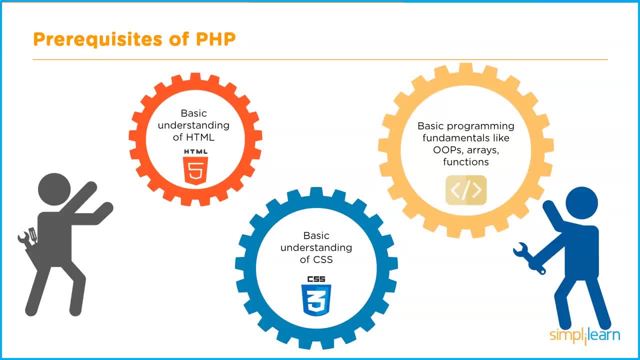 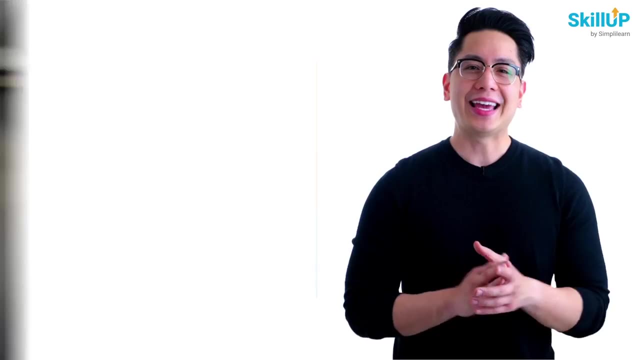 it. It would really help you along the way. Now that we have an understanding of what PHP is, its syntax and how does it function, let's jump to making a first program. If getting your learning started is half the battle, what if you could do that for free? 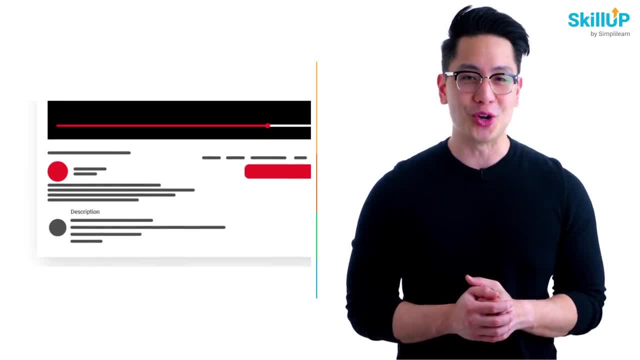 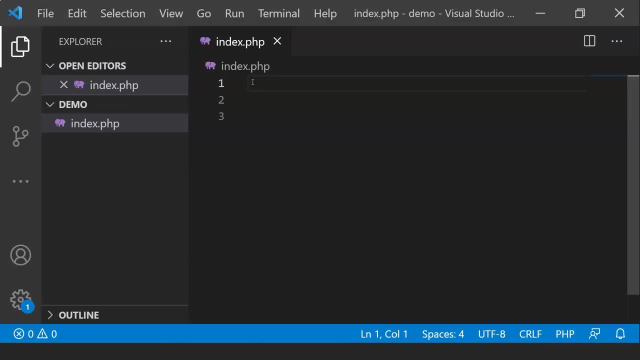 Visit SkillUp by SimplyLearn. Click on the link in the description to know more. Now, since a browser only understands PHP, it's not a problem. It's just a matter of learning. For a browser that only understands HTML, we will write a first PHP script into the. 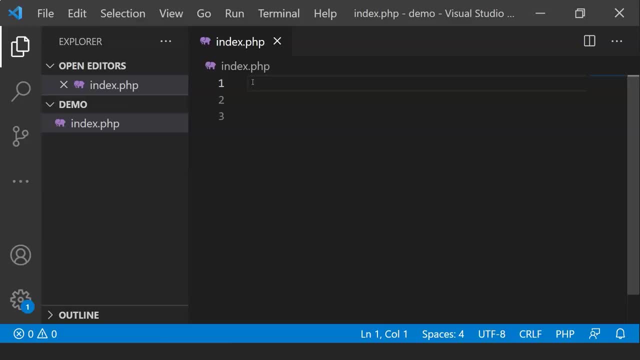 HTML code. So let's get started. I'll begin writing the HTML code with HTMLbody and let us create a first heading. Let's name it firstphpWebPage, the first one. Let's get started. It should look like this: 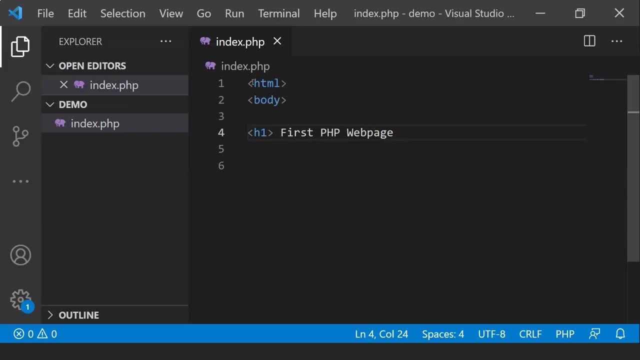 FirstphpWebPage. Ok, let's add that first heading. Next let's name it firstphpWebPage. Now let's write a first PHP script. So a PHP script, as we discussed earlier in the syntax section, begins with an opening.